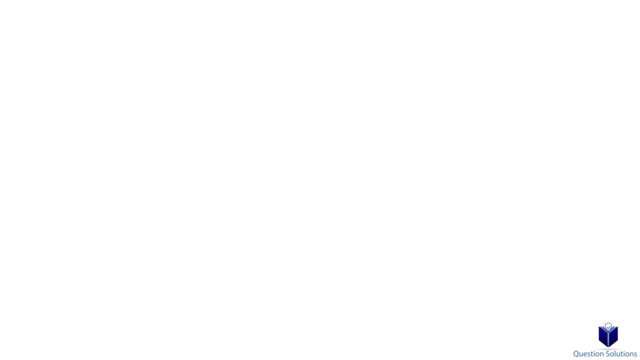 In the previous chapters you probably learned that we can write f equals ma with respect to rectangular coordinates and normal and tangential coordinates. In this chapter we write f equals ma with respect to cylindrical coordinates, So we can say forces added together in the radial axis. 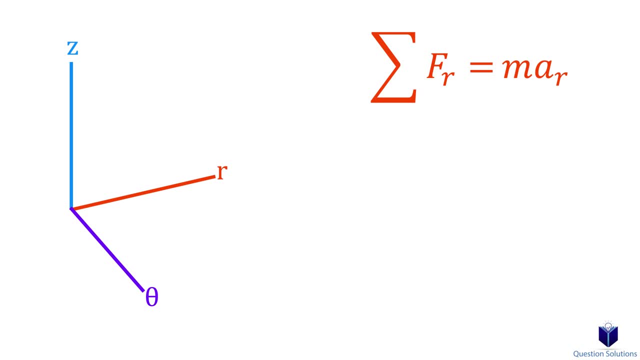 is equal to mass times. the radial acceleration Forces added together in the transverse axis is equal to mass times. transverse acceleration And forces added in the z axis is equal to mass times. acceleration in the z axis. Let's review the basics first. Imagine there is a particle. 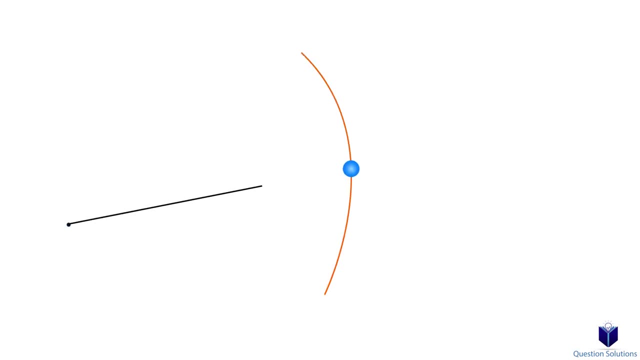 moving along a path From a fixed point, we can say the location of the particle by drawing a radial coordinate. If we then draw a fixed line, we can show the angle with respect to the radial coordinate using the theta symbol. This should be familiar to you. If not, please check the. 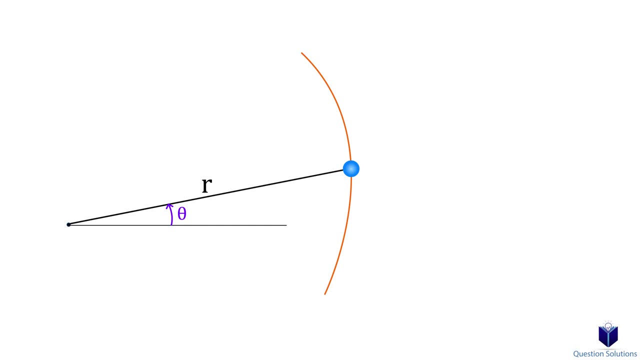 description below for the basics of cylindrical components. The new part we look at in this chapter is when a force is applied to the particle. If the force is applied to the particle, we can see that the force is always perpendicular to the tangent of the path. When we apply a force, 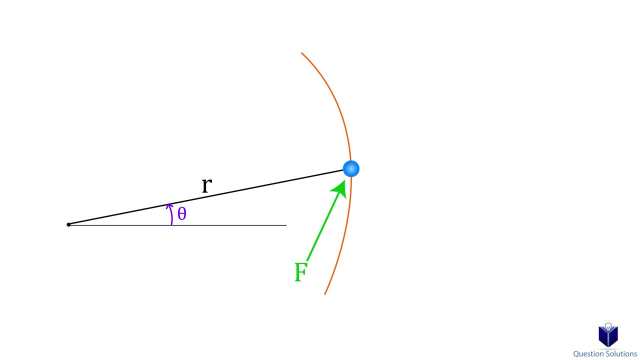 like that. there needs to be a normal force. But the question is: where does the normal force affect the particle? The normal force is always perpendicular to the tangent of the path. So imagine we freeze time and at that location we draw a tangent. Then the normal force is. 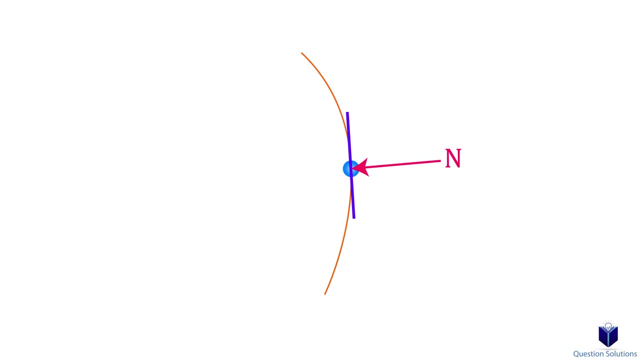 perpendicular to that tangent. The frictional force always acts along the tangent, in the opposite direction of the way the particle travels. In some questions we will need to calculate the force of the particle by drawing a radial coordinate. For this we need to. 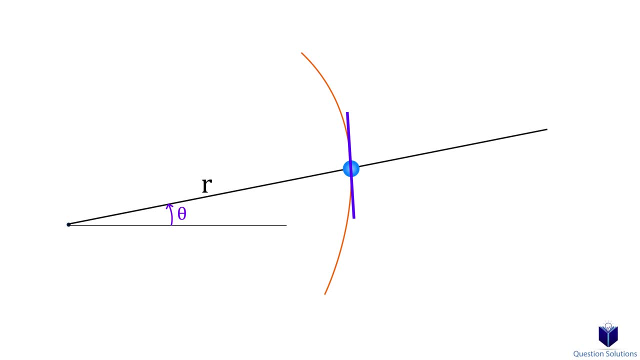 calculate the angle to find the direction where normal and frictional forces affect the particle. For that we use something called the psi angle and it's represented by the psi symbol. To find it we use tan. psi is equal to the radial coordinate divided by the derivative. 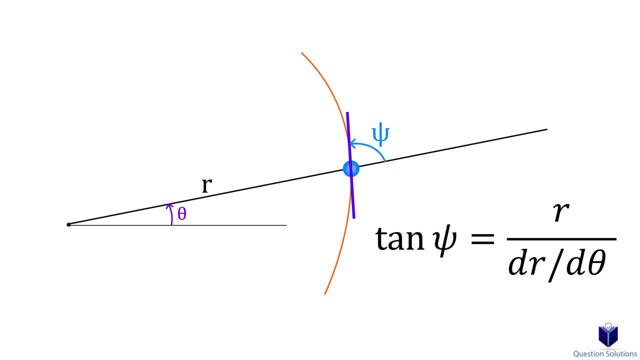 of the radial coordinate. So this angle represents the angle between the tangent and the radial coordinate. There are two possibilities for this angle, which is that sometimes it will be positive and other times it will be negative. If it's positive, all it means is that we're measuring it in the positive direction of theta. If it's negative, 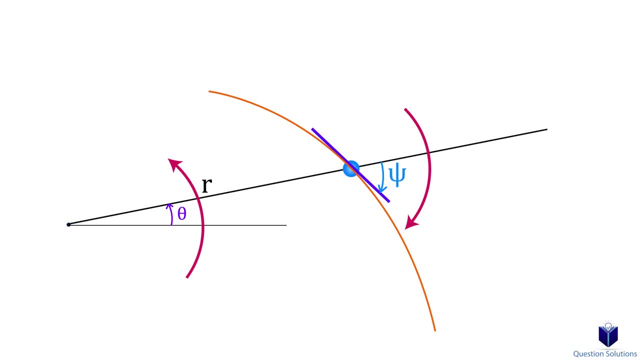 we're measuring from the opposite direction to theta. When we do examples, this will make more sense. Example number 2 in this video uses this angle. Lastly, you should remember how to find radial acceleration, transverse accelerations and acceleration in the z direction using these. 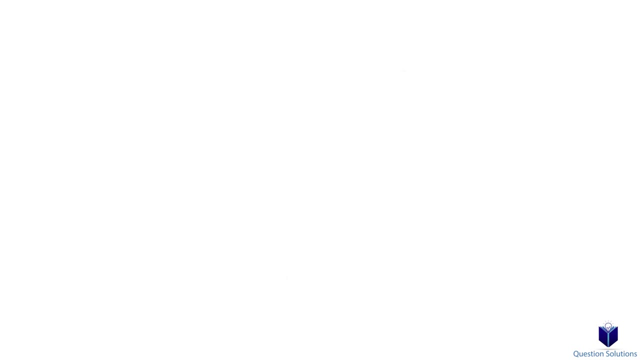 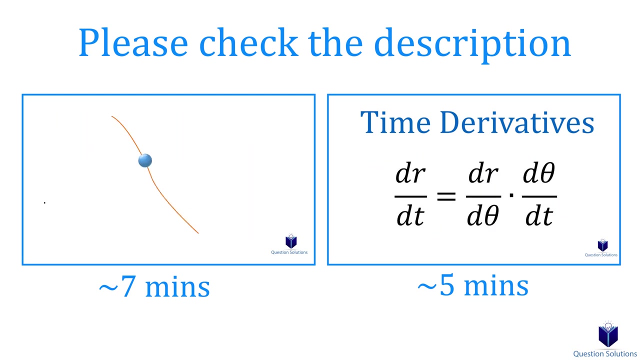 equations And you should remember how to do time derivatives. If you don't remember, please check the description. There are links to videos that goes through these concepts step by step. Let's get started with some examples and by the end you should be able to solve most, if not all, the questions in this chapter. 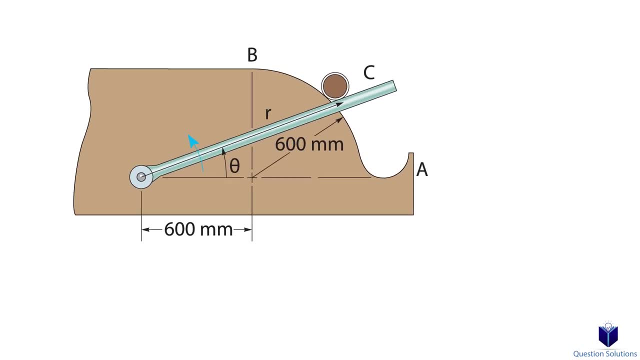 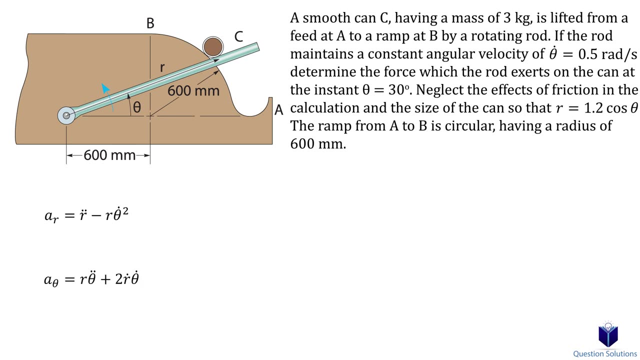 In this question we need to find the force that is exerted on the can. So the first step in these types of questions is to figure out the radial and transverse accelerations. For that we need to use these two equations. Now, from the given information, 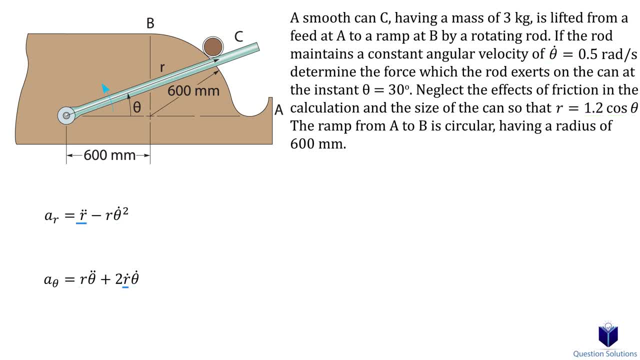 we see that we need the first and second derivative of our radial coordinate And we also have the angular acceleration. So let's do that first. Let's take the first time derivative of our radial coordinate. Now we need to find the force when theta is equal to 30°. So let's plug in 30°. 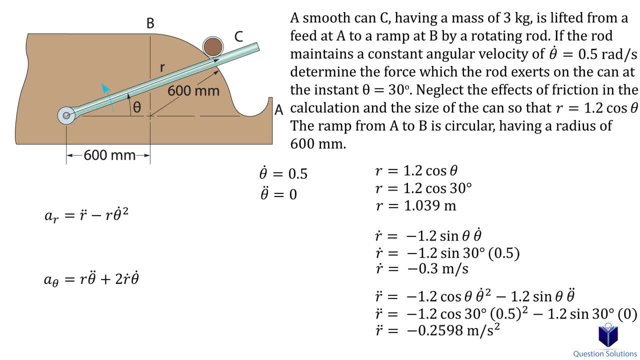 along with the angular velocity and acceleration into our radial coordinate equation equations. Now that we have those, we can find the radial and transverse accelerations. Let's plug in everything we found, first for the radial acceleration, now for the transverse. 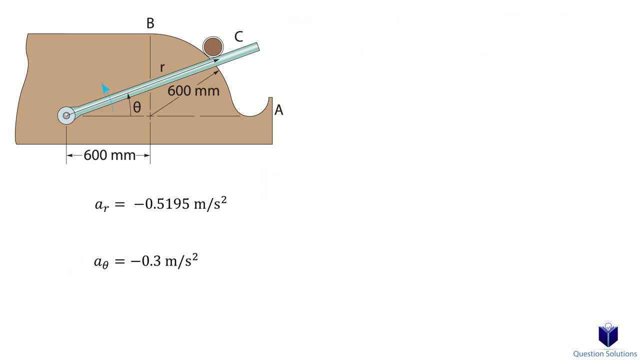 acceleration. Once we have the accelerations, we can move on to drawing a free body diagram. The radial axis will be along the radial coordinate, which means the transverse axis will be perpendicular to it. We see that the force is then applied along the transverse axis. Because this question? 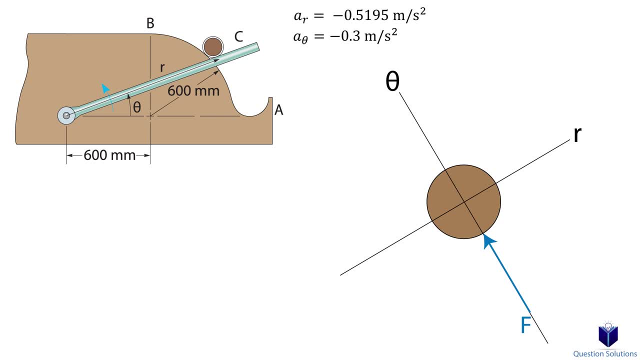 is simple and we're given the angle. we don't need to calculate the psi angle. The weight is straight down, which means it's coming down at an angle of 30 degrees from the transverse axis, and the normal force is perpendicular to the tangent, which means 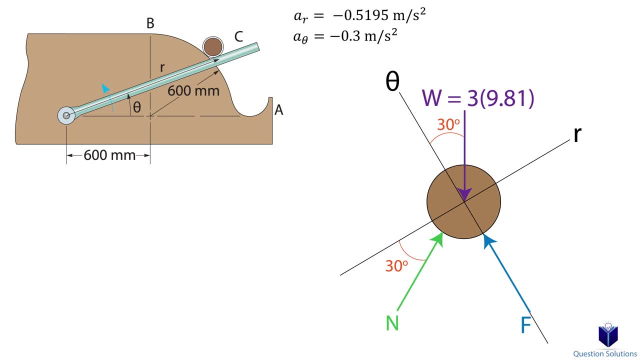 it's coming in at an angle of 30 degrees from the radial axis. Let's write our equations of motion. First, the radial components. So on the left side we have the radial component of the normal force, the radial component of the weight, and that's equal to the mass. 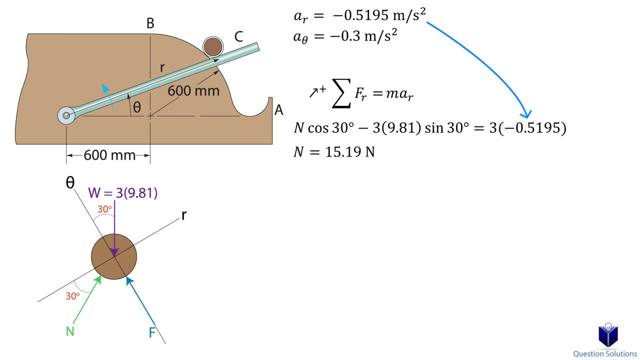 of the can. Let's solve for the normal force. Now we can write an equation for the transverse components. On the left side we have the force, the transverse component of the normal force, which we just found before, and then we have the transverse component of the weight, and that is equal. 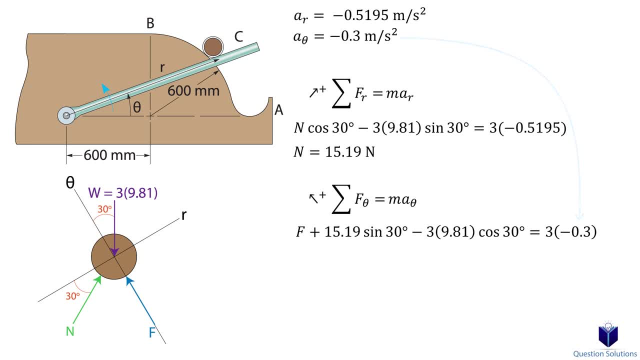 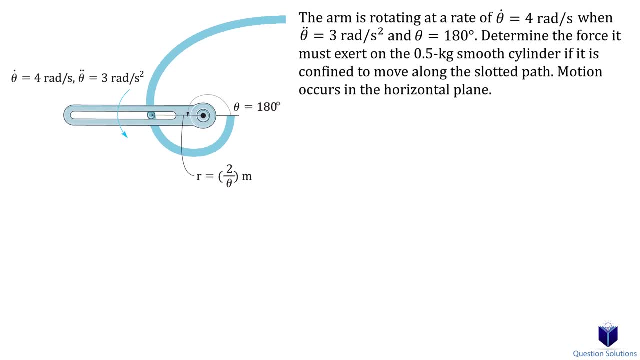 to mass multiplied by the transverse acceleration. Let's solve for the force, and that's our answer. Let's take a look at this example. In this question, we need to find the force required to move the cylinder along the slotted path. So, as usual, our first step is to find 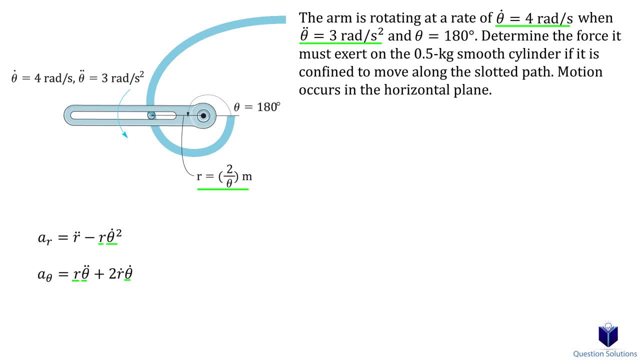 the radial and transverse accelerations. Looking at the information given to us, we need to find the first and second derivatives of our radial coordinate. So let's do that. Remember: one over theta is the same as theta to the power of negative 1.. Let's find the first. 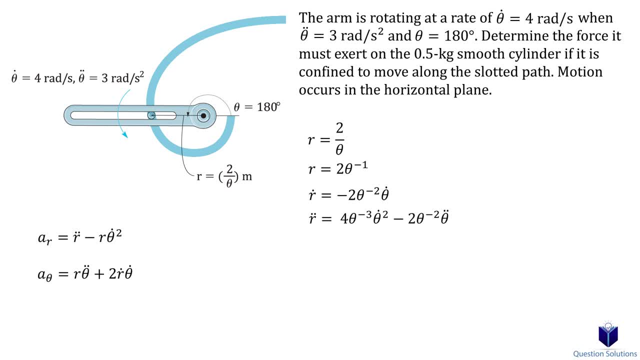 time derivative. Now the second time derivative. So the question says we need to figure out the force when theta is equal to 180 degrees. dick cooled computer don'tteenth degree. rubik's paper. rubik's paper. We need to make sure we convert 180 degrees into radians before plugging it in. 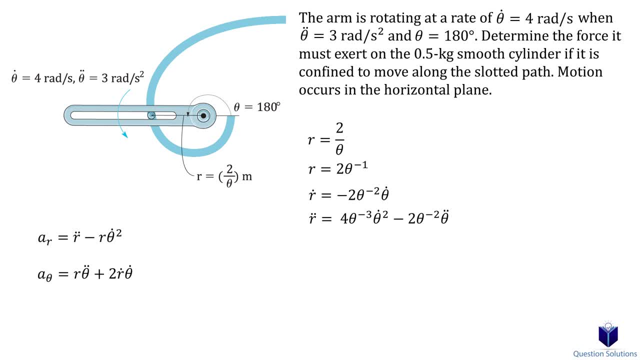 A rule of thumb: if a question doesn't say whether the radial coordinate is in radians or not, check to see if there is a trigonometric terminal like sine or cosine. If it does, you don't need to convert degrees to radians. otherwise you do. 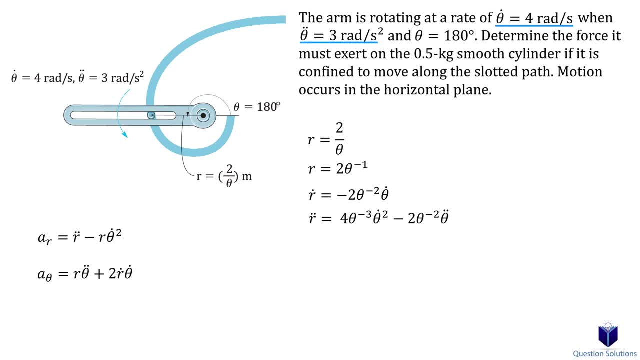 Also note that we're given the angular velocity and angular acceleration in the question. Let's plug in the values and solve. Now we can figure out the radial and transverse accelerations. First the radial acceleration, Now the transverse acceleration. Remember how we talked about the psi angle that sometimes we need to find? 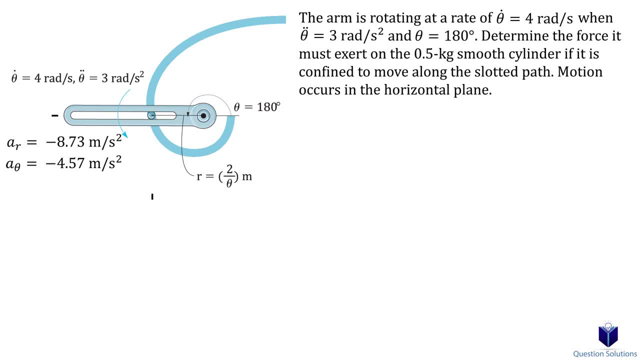 Well, this is the question where we need to find that. To see this visually, let's draw a free body diagram. So first we draw the tangent line, Now the psi angle gives us the angle between the radial line and the tangent line. 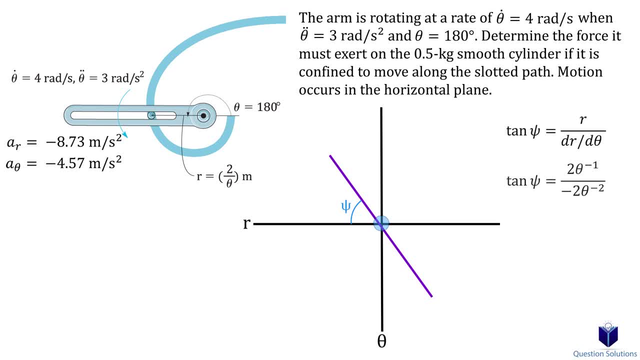 Let's use the equation we learned to figure it out. So on top we have the radial coordinate, On the bottom we have the derivative of the radial coordinate with respect to theta. Remember, this is not a time derivative. Let's plug in theta, which is equal to 180 degrees, or in radians, it's pi. 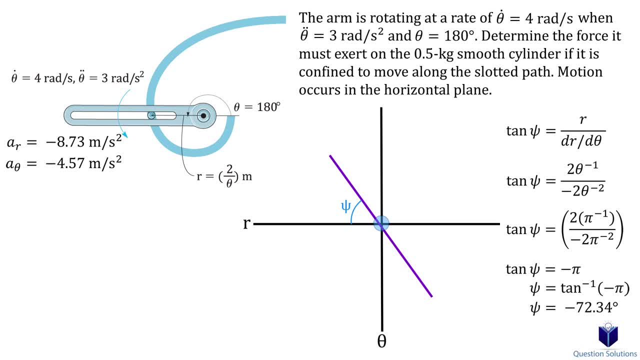 Let's simplify. We got a negative value, which means we're going opposite to the positive sense of theta. So how does this value we found help us? For that we need to draw the normal force. Remember, normal force is always perpendicular to the tangent line. 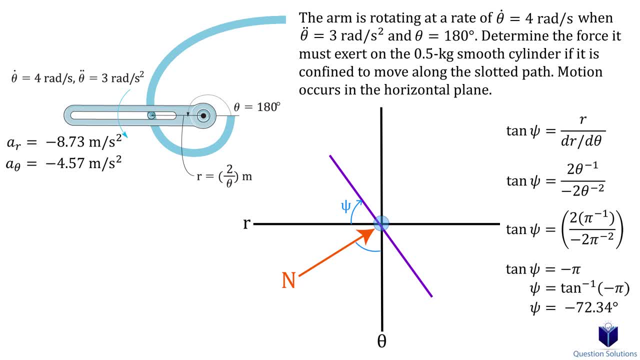 If you look carefully, the angle between the transverse line and the normal force is equal to the angle between the radial line and the tangent line. If you extend the normal force upwards, you can see how this angle is the same. Let's draw the force applied to the can as well, which completes our free body diagram. 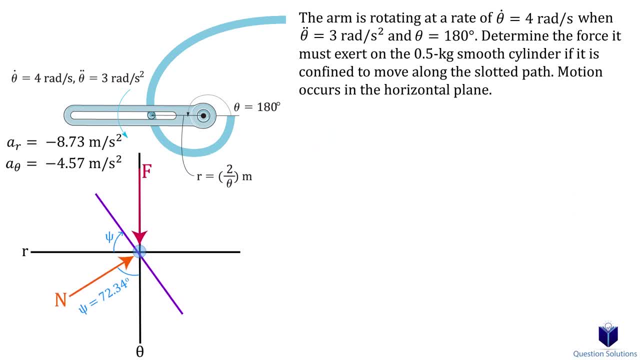 Now that we have the angle, we can finally write our equations of motion. First, for the radial components, We will assume forces to the left to be positive. So on the left side we have the radial component of the normal force and the force applied. 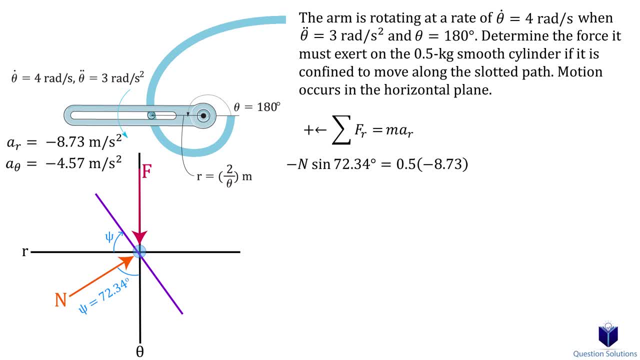 to the can as well. And on the right side we have the mass multiplied by the radial acceleration. Now an equation for transverse components. We will assume forces down to be positive. So we have the transverse component of the normal force which we found before, plus. 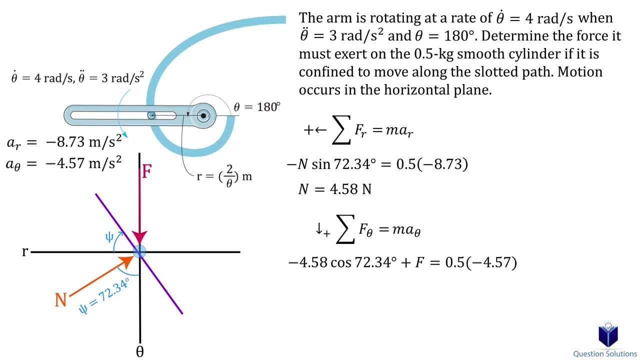 the force being applied by the arm, and that's equal to mass times, the transverse acceleration. We got a negative value, but that just means that instead of the force coming down from the top, as we drew on the diagram, it's coming from the bottom. 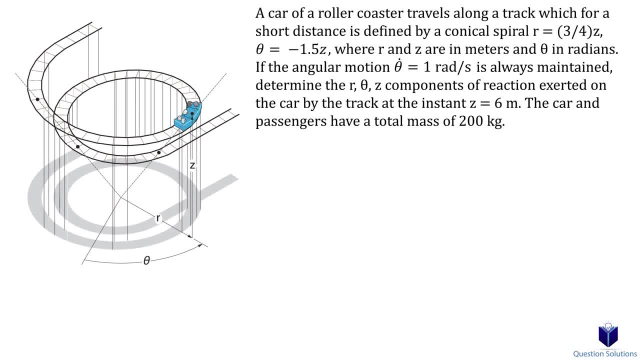 And that's our answer So far. we looked at a normal F equals ma question with cylindrical components and another question where we had to calculate the psi angle. For our last question, let's look at an example where we consider the z-axis as well. 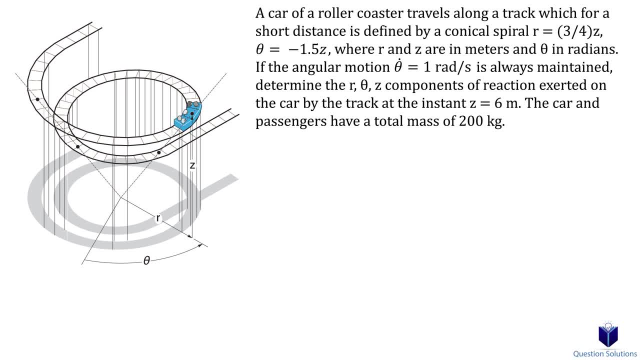 In this question we need to find the radial transverse and the z-forces exerted on the car by the track. So, in simple terms, we're looking for fr, f, theta and fz. In this question we're looking at the path of the roller coaster. So, in simple terms, we're looking for fr, f, theta and fz. In this question we're looking at the path of the roller coaster. So, in simple terms, we're looking for fr, f, theta and fz. So, in simple terms, we're looking at the path of the roller coaster. 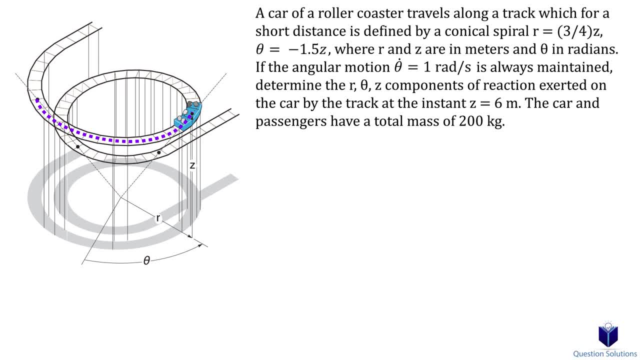 From this point to this point. Knowing this makes it easier to understand how the radial coordinate is represented. The radial coordinate for this question is given with respect to the z-axis, in other words height. As always, we need to find the radial and transverse accelerations, but for this question 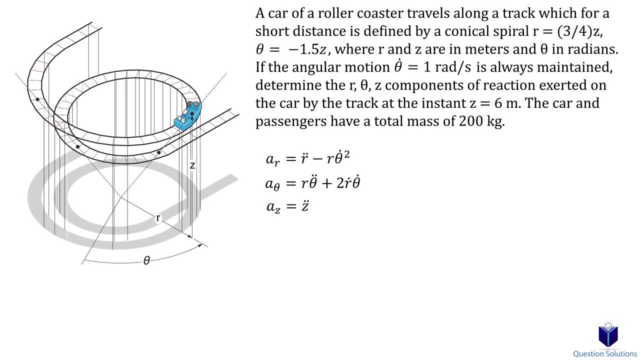 we also need the acceleration in the z-axis. So these are the equations for those, which means we have a few things to find before we can plug anything in. We will start off with the time derivative, the derivatives of the radial coordinates. Now we need to find the angular velocity. 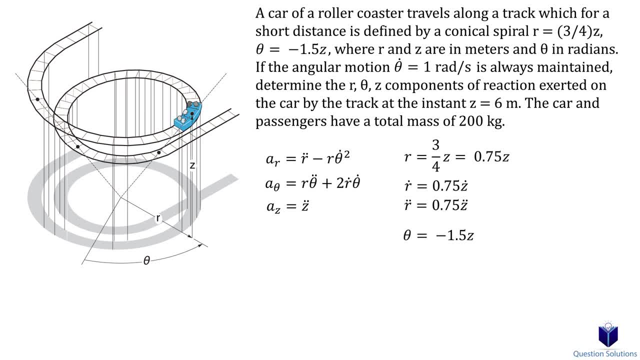 and acceleration. We're given the angle with respect to the z-axis as well, so let's take the time derivatives. Now for the z-axis derivatives. In the question we're told that an angular motion of 1 rad per second is maintained constantly. So what if we substitute 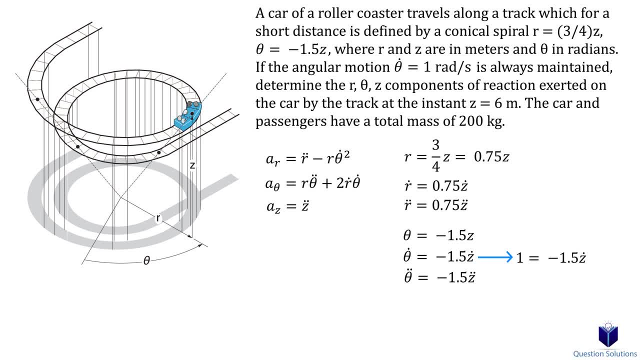 that value into our angular velocity, Then we can solve for the derivative of our z component, In other words the velocity in the z-direction. If we take the derivative of this again, we can get the acceleration in the z-direction. Since the velocity is constant, the acceleration 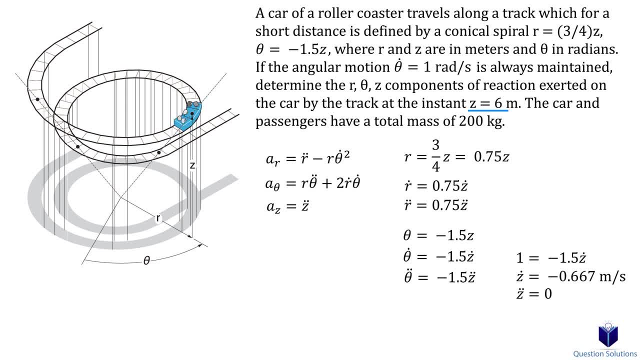 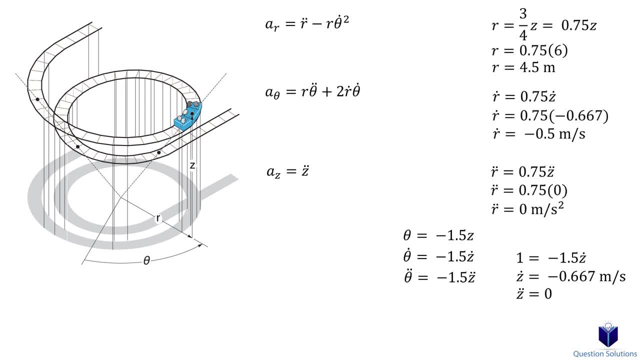 will be 0.. Now we're going to look at the instant when z equals 6 meters. And we found the velocity and acceleration, so let's plug them into our equations. Now we can find the three accelerations. We'll start with the radial acceleration. Remember to plug in the 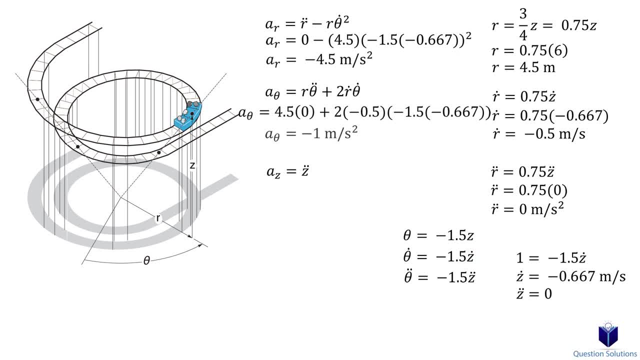 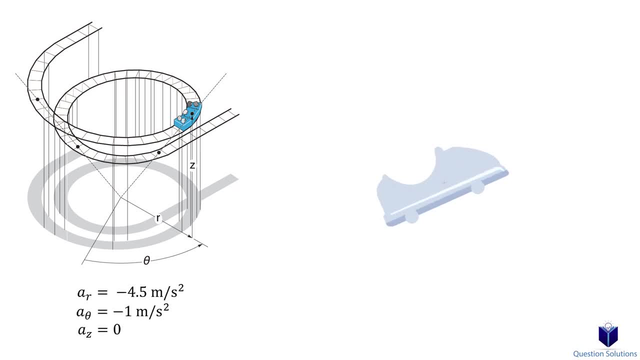 z velocity as well. Now for the transverse acceleration. Here you'll notice that there are times when you can use brute force. You can also. Lastly, the acceleration in the z direction is zero. Let's draw our free body diagram. We have the force in the radial direction, the force in the transverse direction, the 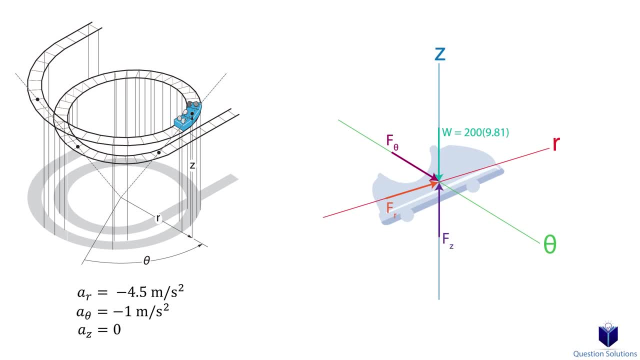 force in the z direction and we have the weight. Let's write our equations of motion. First for the radial direction. the only force we have in this direction is the radial force, so that's equal to mass times radial acceleration. Let's solve for the radial force. 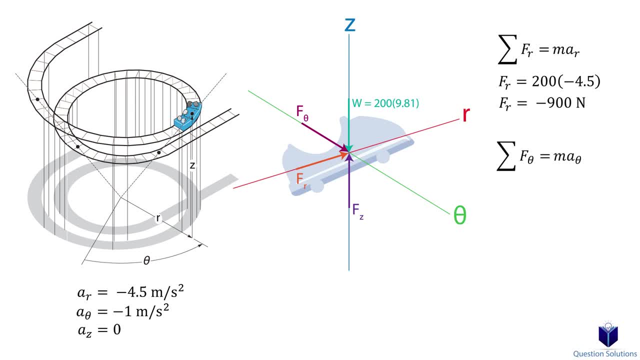 Now an equation for the transverse direction. Again, the only force in the transverse direction is the transverse force, so that's equal to the mass times, the transverse acceleration. Lastly, let's write an equation for the z-axis forces.